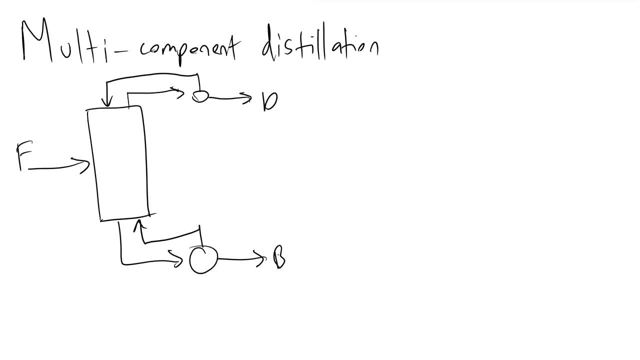 take out a bottoms stream and the put some of our freight back into our distillation column and then we'll put a. this is going to be the same type ofultural system that we saw earlier. The first thing to do when you are given a multi-component distillation problem is make a table to have. 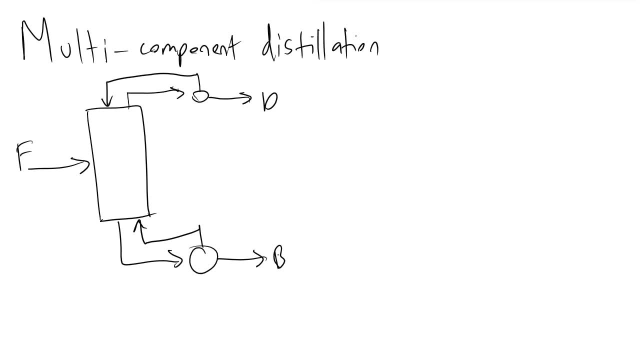 all your components and list them in terms of the, with the most volatile component at the top and the least volatile component at the bottom. In other words, you will have the component with the highest boiling point at the very top of your table and the lowest boiling point at the bottom. 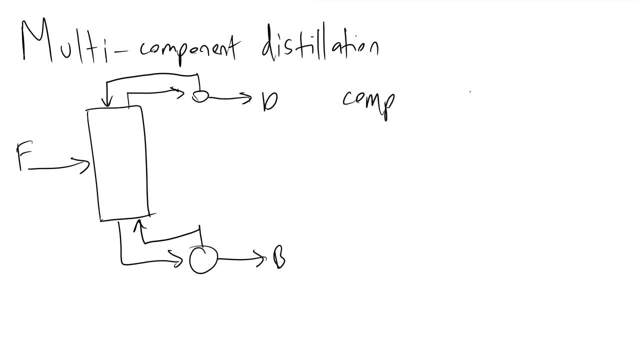 table I will have a column for a component and then I will define another quantity, alpha i, hk, And this tells us the relative volatility of component i to component, to our heavy key component. that I'll get to in a few minutes or seconds. 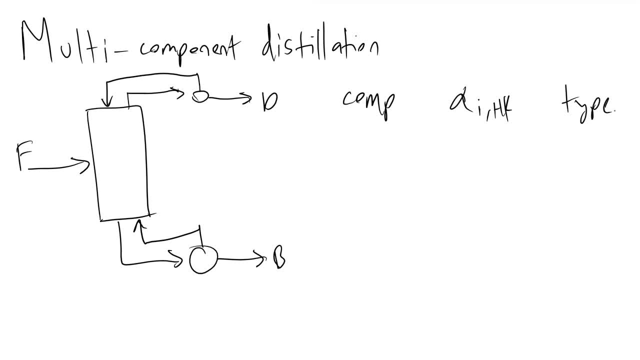 And I'll have another column here, just so that we can keep track of what type of component, which I'll get to in a little bit. So in this generic example, I'll be having four components: a, b, c and d. 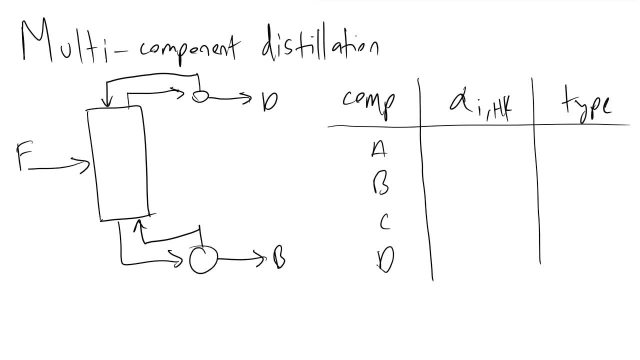 And I will define component b as what we call a light key and component c as a heavy key. And the reason we need to define heavy keys and light keys is for the mathematical models that we'll apply later on And when we are deciding what two species to declare as our heavy and light key. it 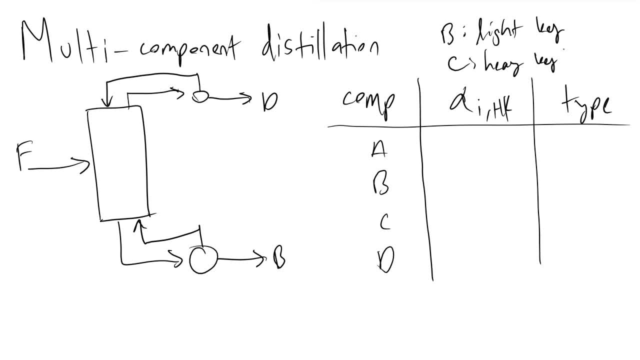 is best to pick two components that have the biggest difference in volatility or boiling points, And the greater the difference between these volatilities of these two components, the better our non-distributing assumption that we'll make later on becomes. And so, in this example, because I let component b be our light key and component c be our heavy, 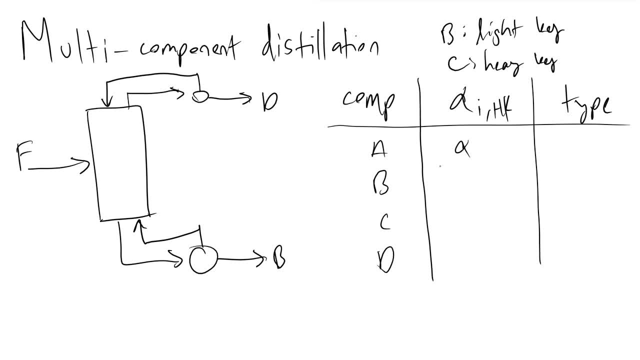 key what we'll have and you'll have numerical values when we were actually evaluating problems like this. but in this example we have alpha a- hk, and that would have some numerical value. we have alpha b- hk, and then the relative volatility of the heavy key to the relative volatility of 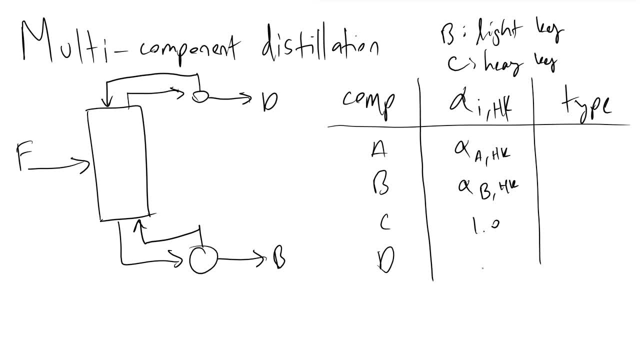 the heavy key, we'll have a value of 1.0, and then, finally, we'll have a relative volatility of component d to the heavy key here. And what a further note I would like to make at this point is to recognize where or what. 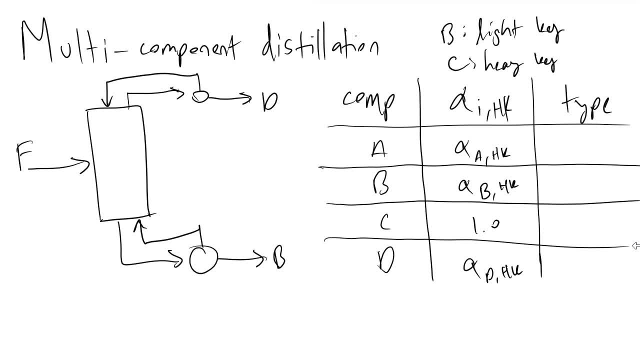 type of components these are, And so we already defined that component b was our light key and component c was our heavy key, And what that means is that we'll have additional types of components. Anything above your light key on this table that we've just drawn will be referred to. 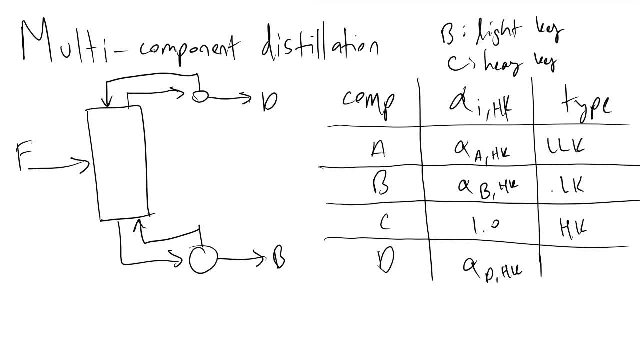 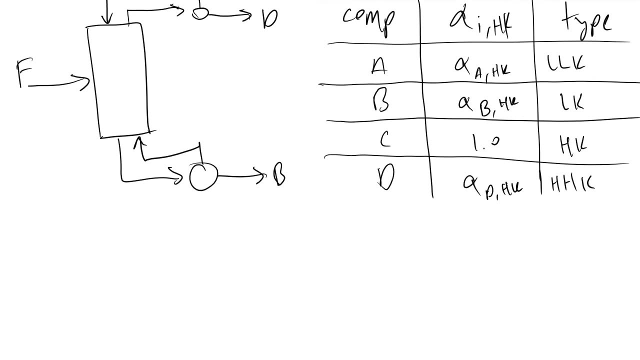 as a lighter-than-light key component. so LLK and anything beneath the heavy key on this table will be referred to as the heavier-than-heavy key component. And the next step that we will make in modeling our system, is to say, is to make the non-distributing 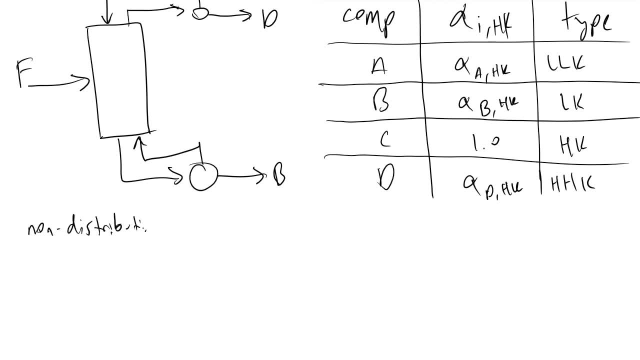 assumption, And what the non-distributing assumption tells us, is that all lighter-than-light key components from this table that we just drew will only exit our system in the distillate And all heavier-than-heavy key components will only exit in the bottoms stream. 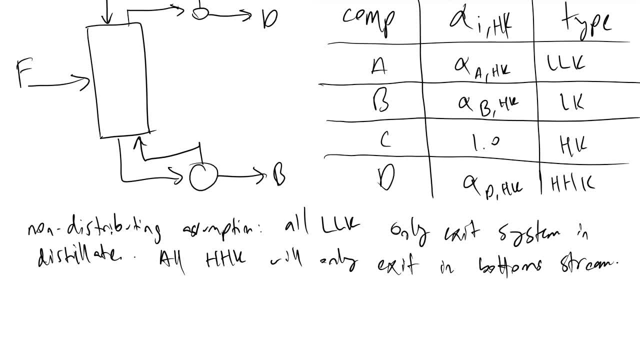 And the reason we make the non-distributing assumption is that it allows us to make mass balances. If we do a component mass balance on a heavier-than-heavy key, we're able to generate some equations that help us define variables or solve for variables later on. 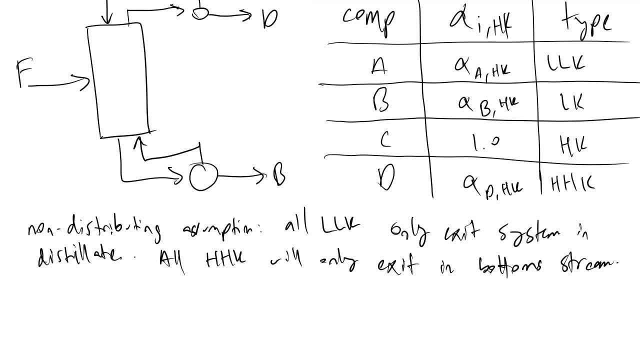 And to go over, a key point to take away before we define a light key and a heavy key in our example is: we would want, in our generic example, αBHK or αLKHK to be a lighter-than-light key component. 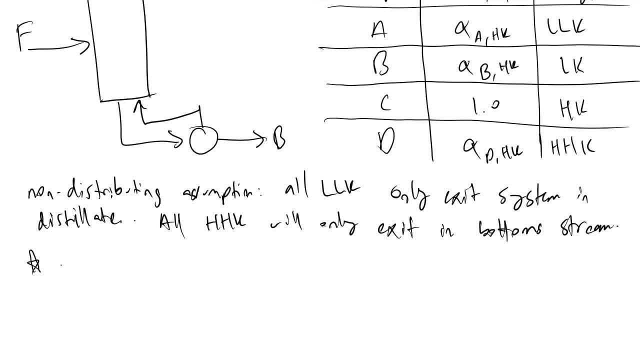 So we want αLKHK to be as much greater than 1 as we can make it, because it makes the non-distributing assumption a better approximation. And at this point a good question to ask is how many trays will be required in our 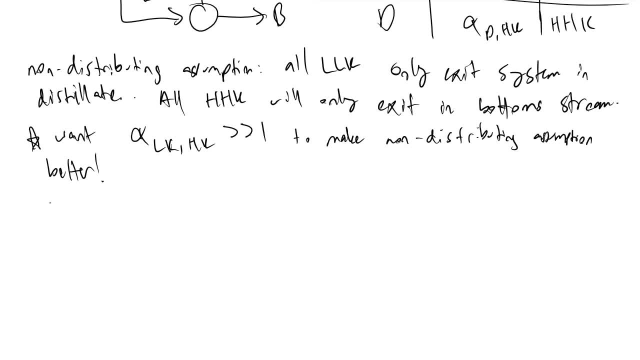 multi-component distillation unit, And so we'll have some requirements, such as: we want a certain concentration of some particular component in our distillate stream, And The way we'll do that is we'll turn to something called the Fenske equation, spelled F-E-N-S-K-E. 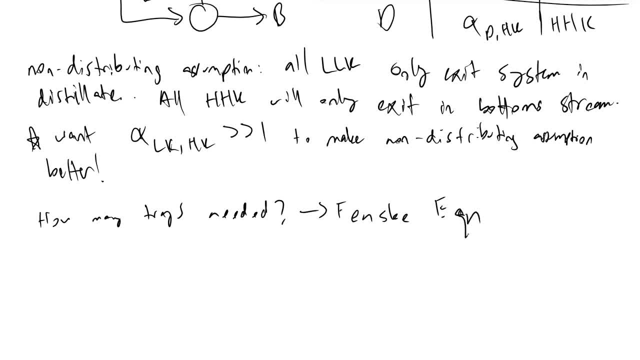 The Fenske equation tells us that: N. the number of trays that will be required is equal to log base 10 of the quantity Of the, Of the, Of the molar ratio of our light key or distillate, divided by the molar ratio of our heavy key. 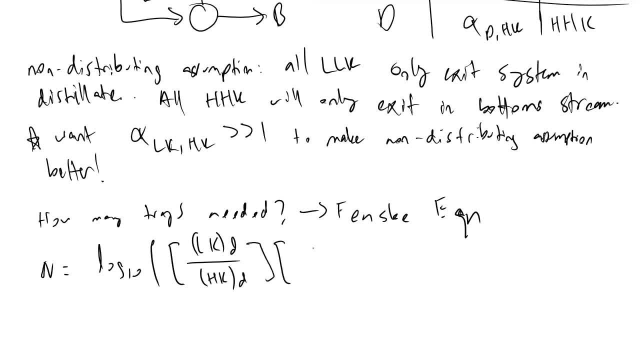 or distillate Times, the molar ratio of our heavy key and our bottom stream divided by the molar ratio of our light key and out bottom stream. And we divide this first Or This logarithm by the logarithm Of our 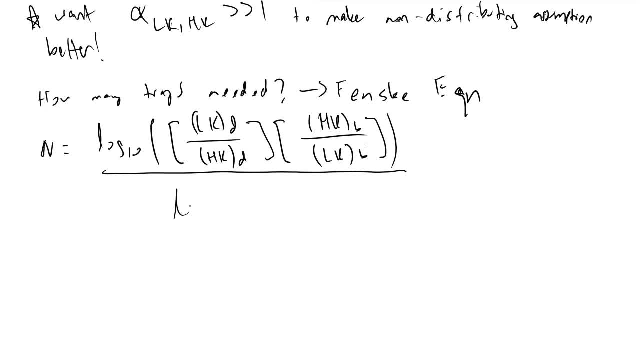 then this is log base 10, of alpha, so the relative volatility average, And so the first thing I'll do is note the terms inside of this top in our numerator. This is the mole ratio of the heavy component in the bottom stream And something to 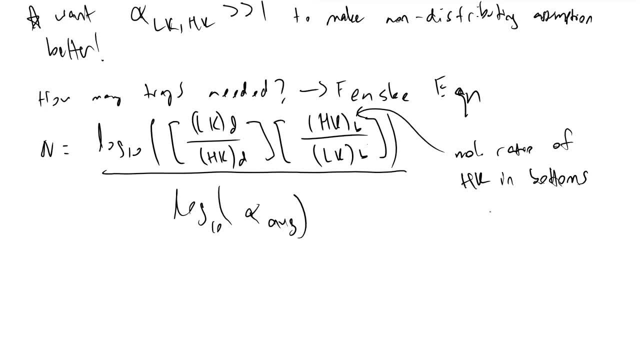 understand is that, because our heavy key is less volatile, it will be more concentrated in the bottom stream than in the distillate, And it'll be a lot more concentrated than the light key in the bottom stream, And so we would expect both of these quantities inside of our logarithm function to be 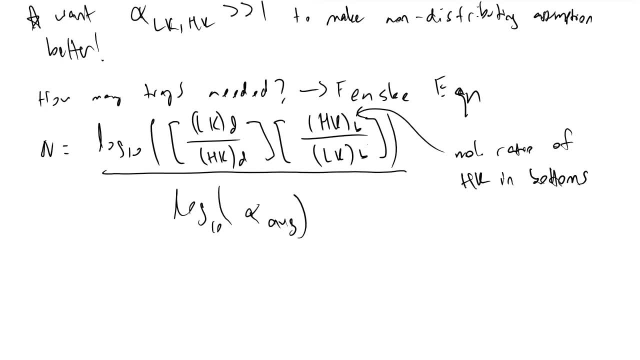 greater than 1.. And what this alpha average term is is a geometric mean of the relative volatility between your light key and heavy key, evaluated at the top and the bottom of our column. And it's important to note that inside these distillation columns, 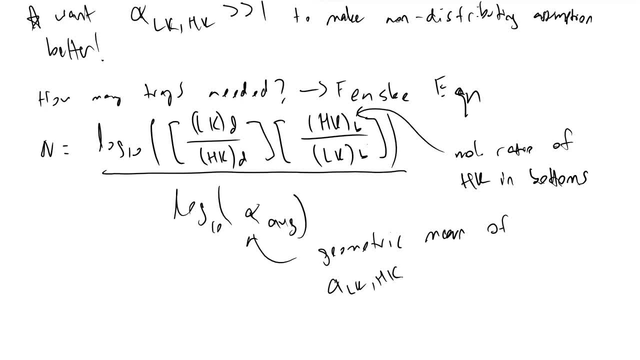 the bottom tray will have a much higher temperature than at the top of the column, and that's because in our reboiler, that's where we're adding in a lot of heat to our system, And at the top of the column, that's where our condenser is. 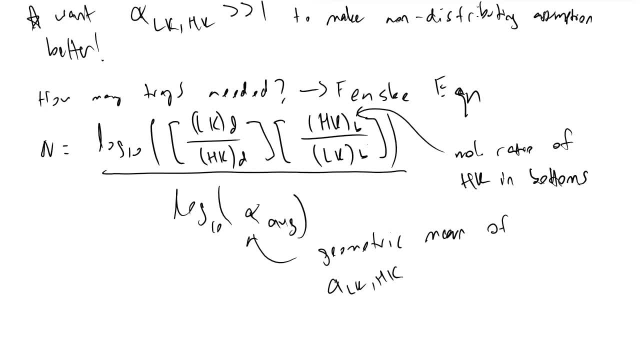 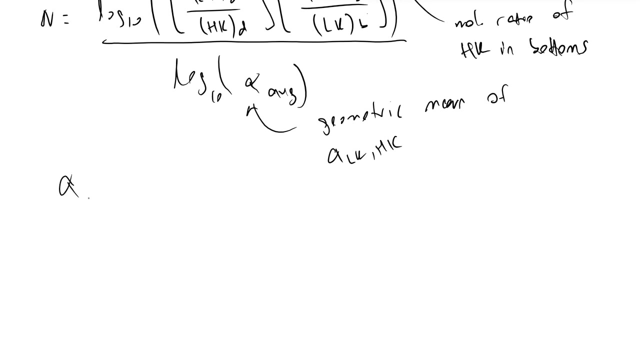 removing heat, heat from our system, so it will naturally be a lot colder and so, because of this, the vapor, the volatilities, will take on a different values, because the volatility will have be some function of temperature that will have to evaluate, and so elaborating on what this alpha average term is is equivalent to the 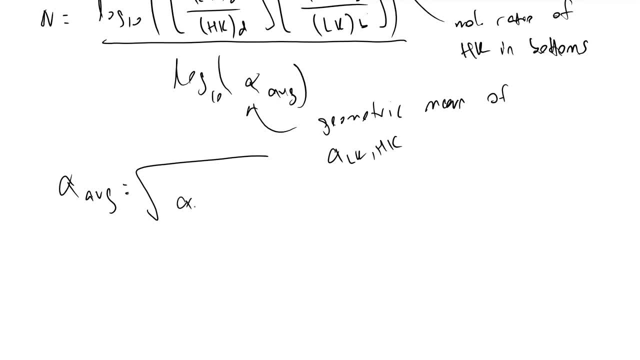 square root of alpha LK. HK, evaluated at the top of the column, divided by alpha LK- I'm sorry you're multiplying it by alpha- the relative volatility of your light key to your heavy key at the bottom of your column. and so these are functions of temp temperature. 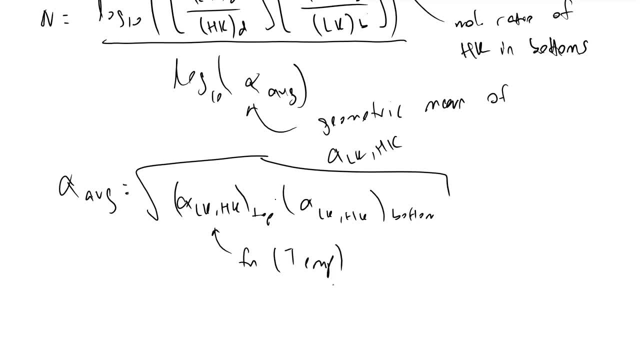 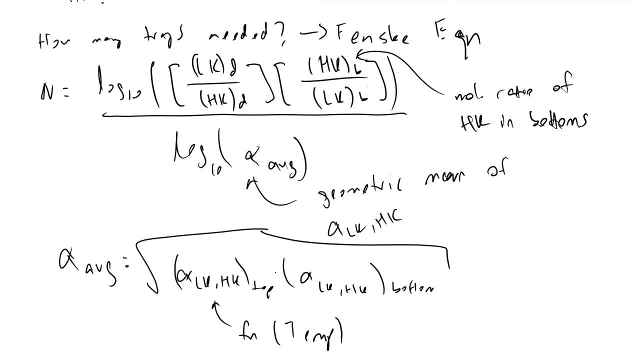 and so once we know what these two terms are, we can evaluate alpha, average and generally in a problem statement, or your supervisor will come to you and I'll tell you that we can't have. we need a certain molar ratio of our light key and a distillate or something like that. we can now fully define the number of.